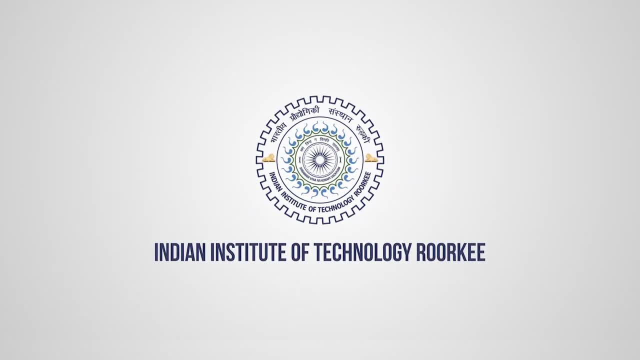 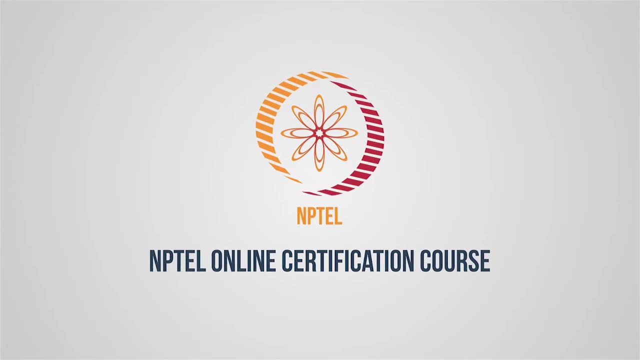 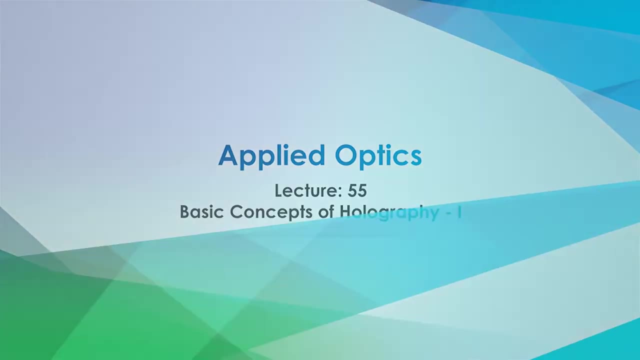 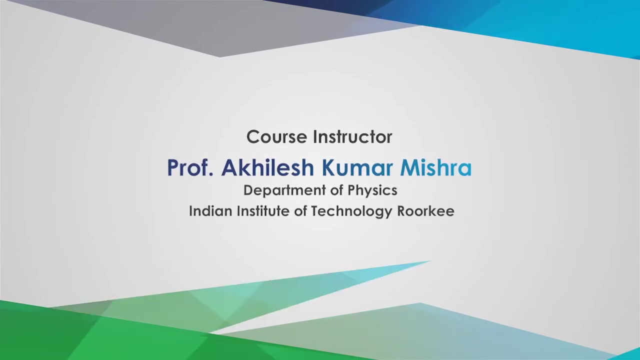 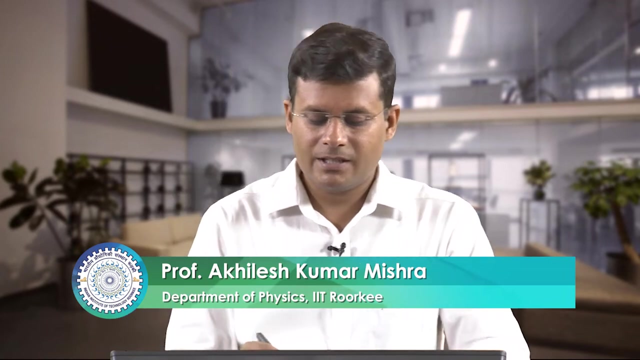 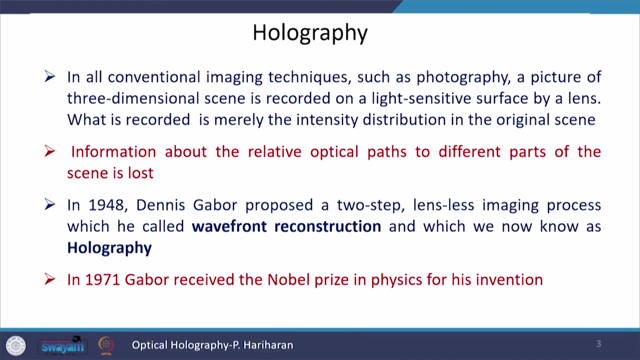 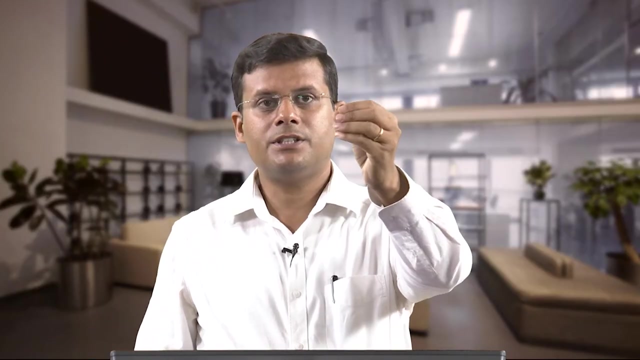 Hello everyone, welcome back to my class. Today we will address the second topic in module number 12, which is basic concepts of holography. You must have seen 3D floating images which if you try to touch then you will see that you are just touching your fingers. it floats in the air but it cannot be touched. 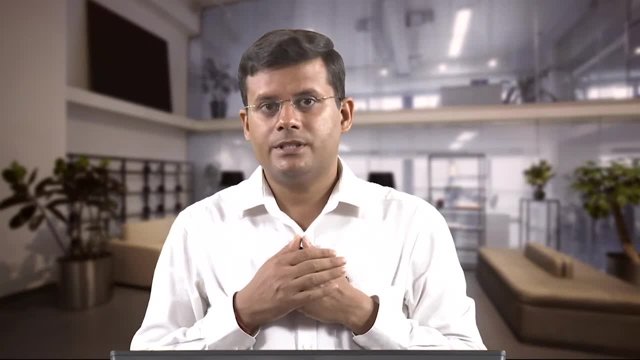 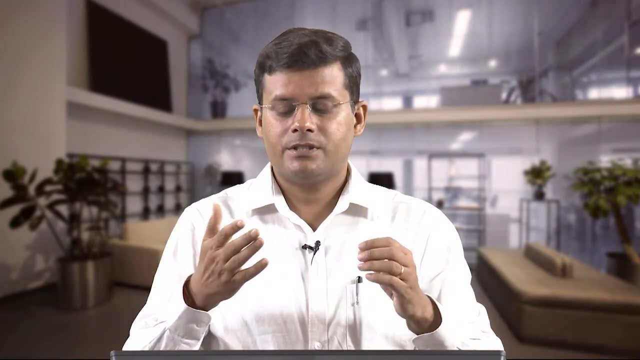 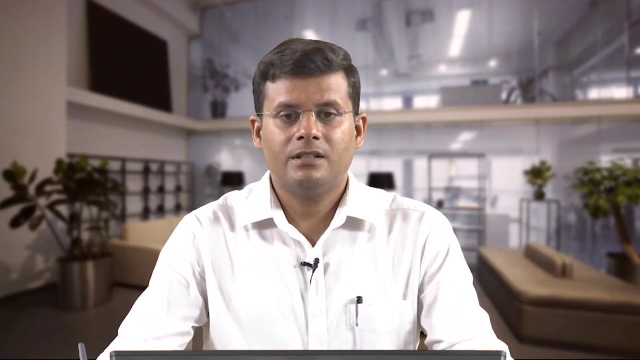 In today's lecture, we will learn how to form these images and what is the drawback of usual images which we shoot using our camera or which we see in the photographic plate? Now, in all the conventional imaging technique, such as photography, a picture of three-dimensional. 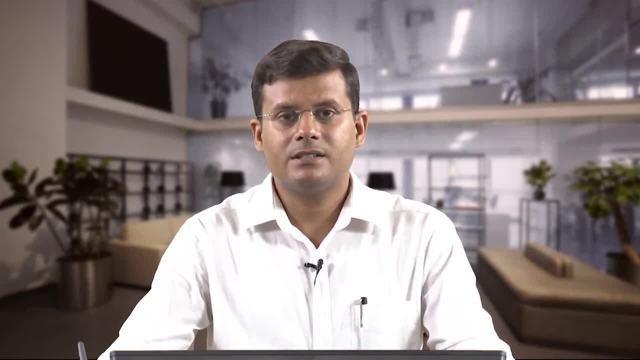 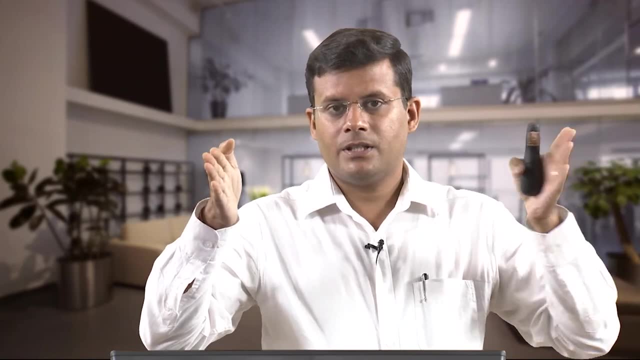 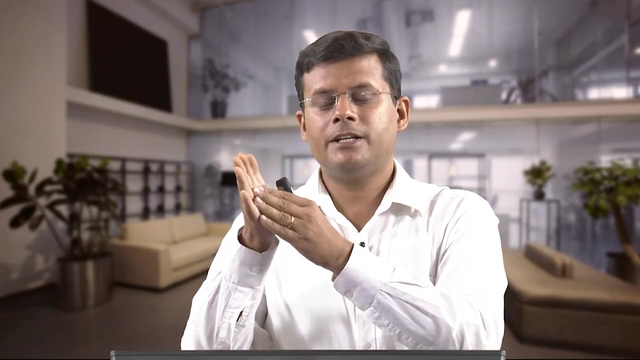 scene is recorded on light sensitive surface by a lens And whenever we record a 3D surface on a 2D surface, then that this 2D information which is recorded on a 3D surface is recorded, which is just the recording of intensity. It does not hold complete information of the 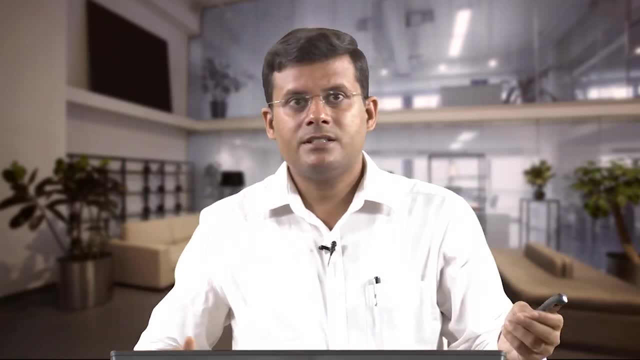 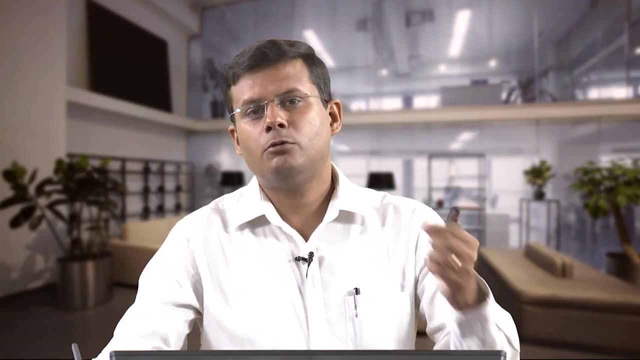 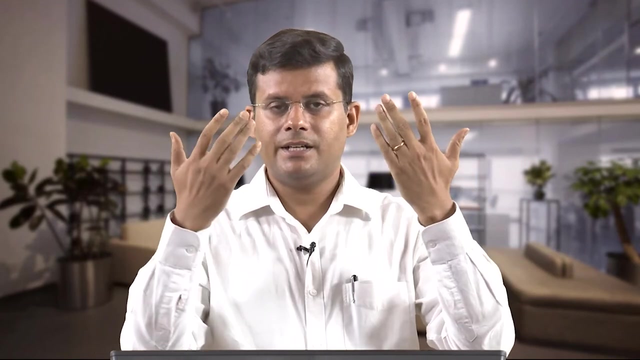 object. What is recorded is merely the intensity distribution in the original scene. We do not record depth. Suppose someone is clicking a photograph of mine, then what will be recorded is the intensity pattern. He will be able to see where my nose is, where my eyes are. 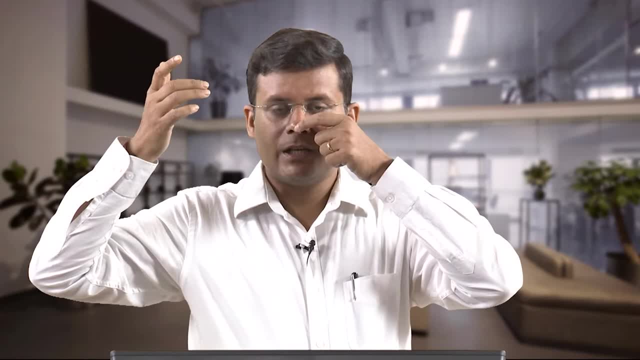 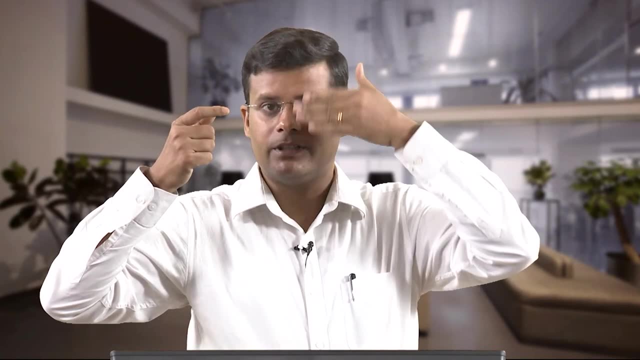 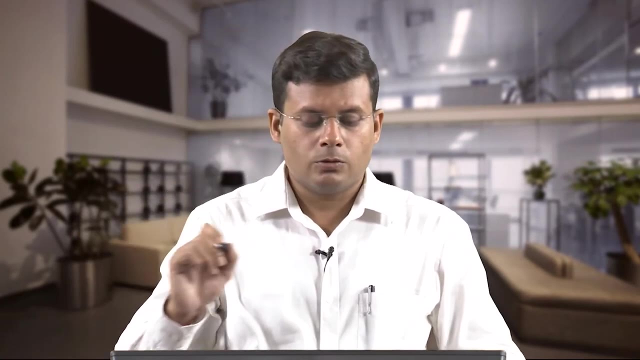 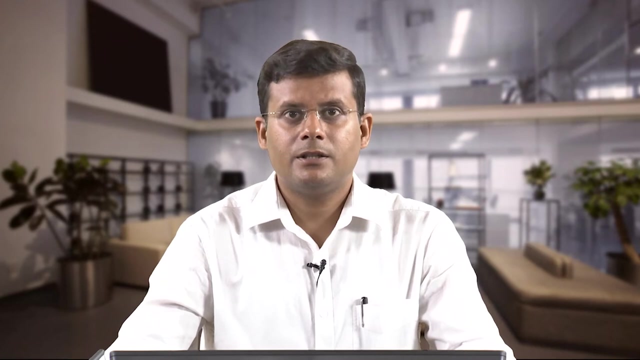 where is my forehead, But he would not be able to clearly say how high my nose is and what is the depth of my eyes from the forehead surface. This depth information would be missing And also, or alternatively, what we can say is that information about the relative optical paths to different 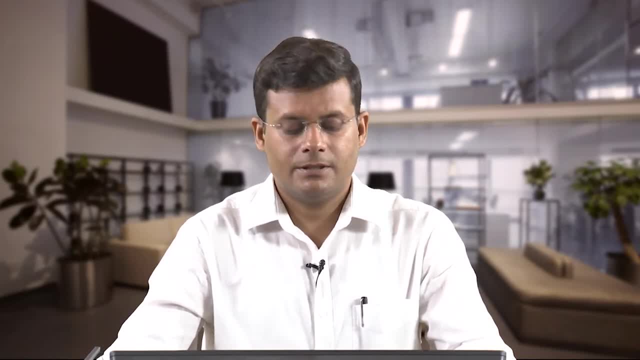 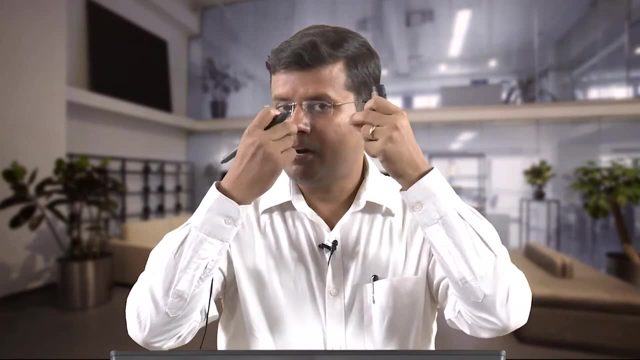 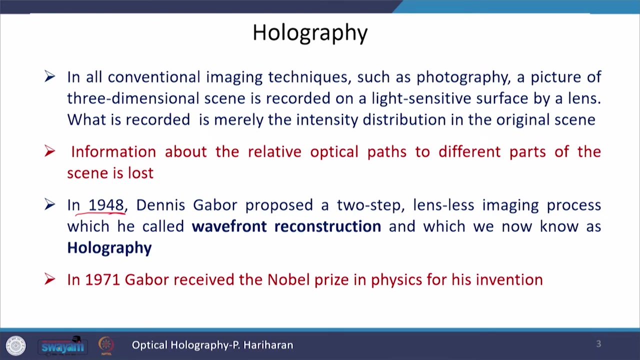 parts of the scene is lost. Yeah, Because ra is coming from my nose and ra is coming from much. Then is there a difference in the optical path lengths? But in 1948, the scientist Dennis Gabor, he realized this And he proposed a two-step. 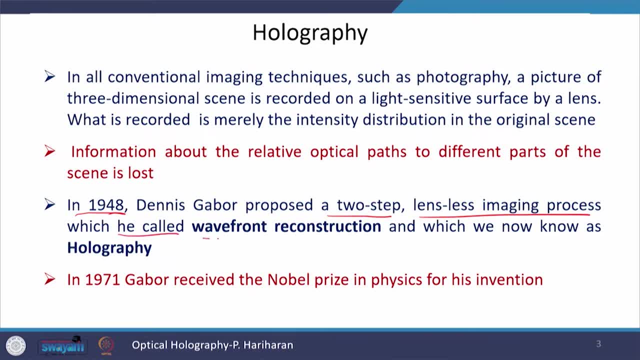 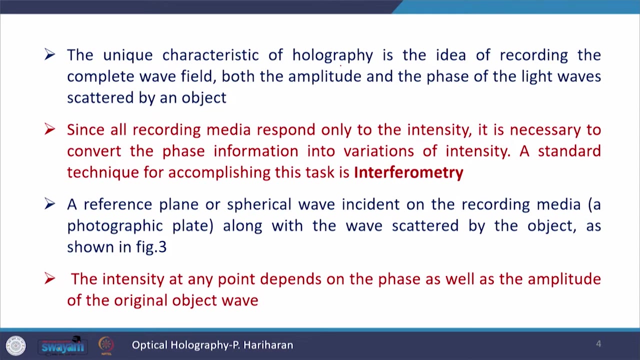 lensless imaging process, which he called wave front reconstruction and which we now know as holography. 3 Runs, 3讲 …. Gabor received noble prize in physics for his invention. Now you can realize how important this technique is. The unique characteristic of holography is the idea of recording the complete wave field. 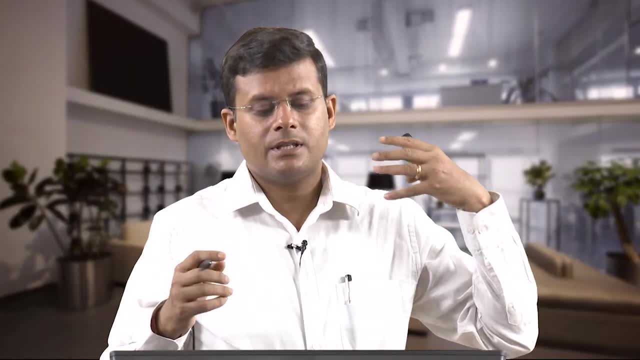 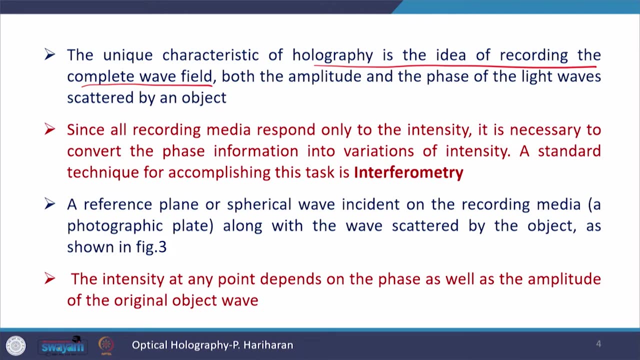 Whenever I say complete, it means it is recording both the amplitude and the phase. Now, since all recording media respond only to intensity, it is necessary to convert the phase information into variation in intensity, Because whenever we record anything, it is just the intensity which we see and record. 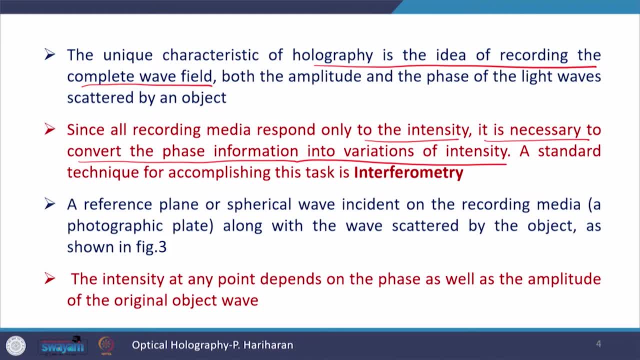 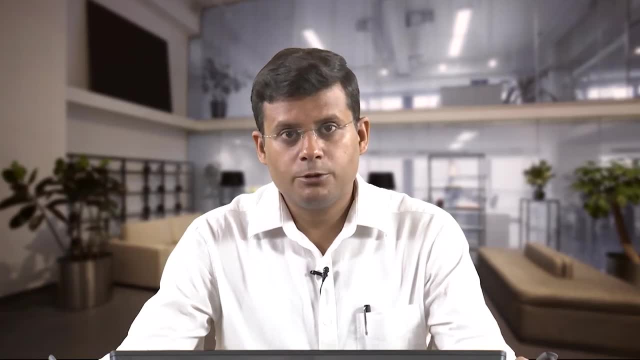 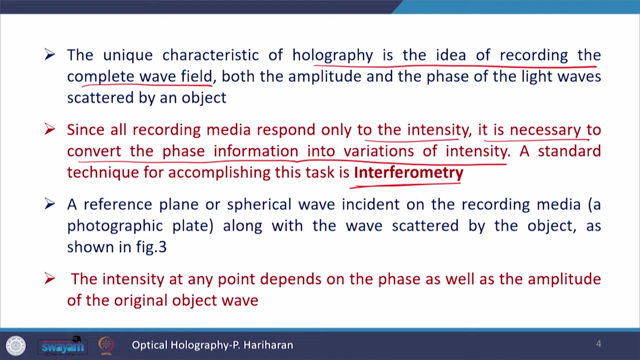 But the phase information is missing. How to feel the phase? The only way is through interferometry. A standard technique For accomplishing this task of changing phase information into intensity fluctuation is interferometry And we know that in all interferometry if you change the phase, the light intensity, 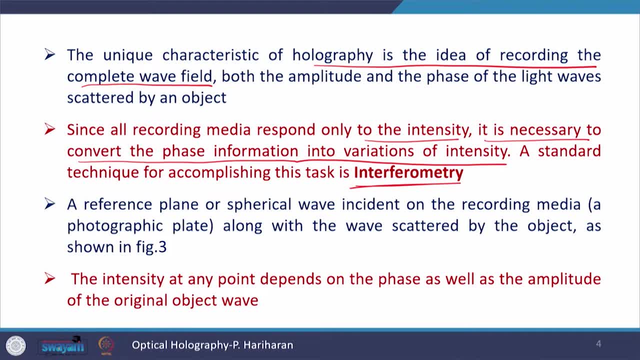 varies and we saw that in interference and diffraction that fringes are formed, And this is only due to the change in phase. Now, what does people usually do using this interferometry? in holography, A reference plane wave or sphere Or spherical wave incident on the recording media, along with the wave scattered by the 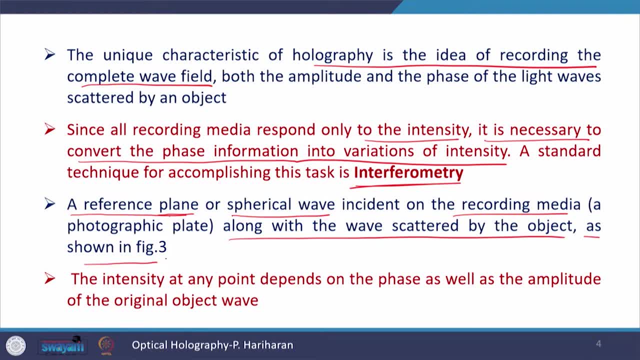 object form: an interferometric setup. I repeat, in an interferometric setup we have a reference plane or a spherical wave that is made to incident on the recording media along with the wave, which get scattered from the object, Okay, And they both fall on some form. 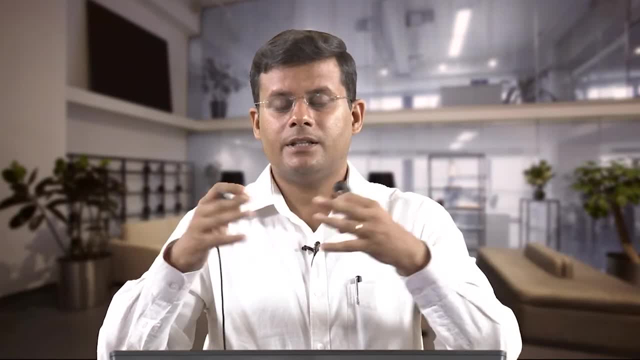 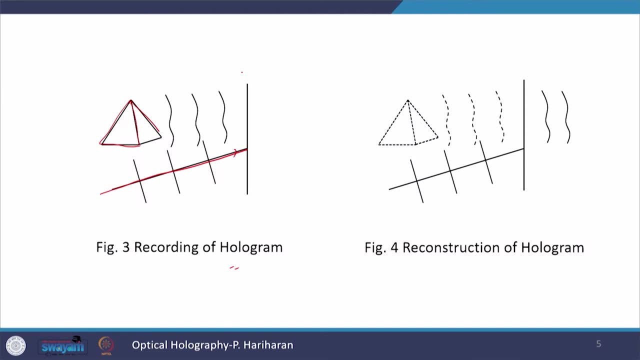 Okay, And they both fall on the photographic plate, They interfere there and then get recorded, And this is shown here in this figure 1.. Recording of a hologram. This pyramid is the object which we want to record on the hologram. 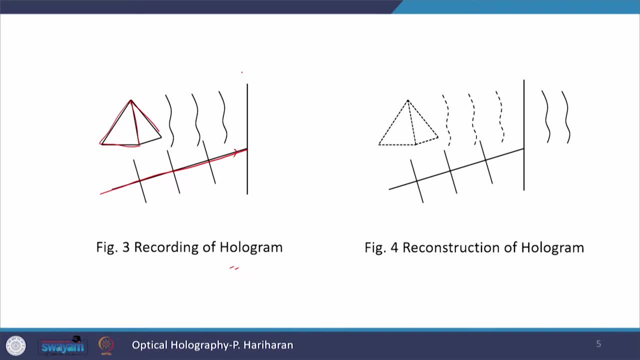 And what people do is that the people launch a reference wave on a photographic plate. This is our photographic plate. Photographic plate Or you can say hologram. Okay, So this is our hologram. Now people launch a reference wave and scattered wave from the object. 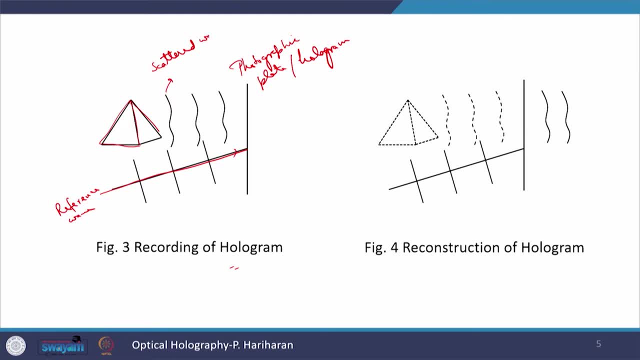 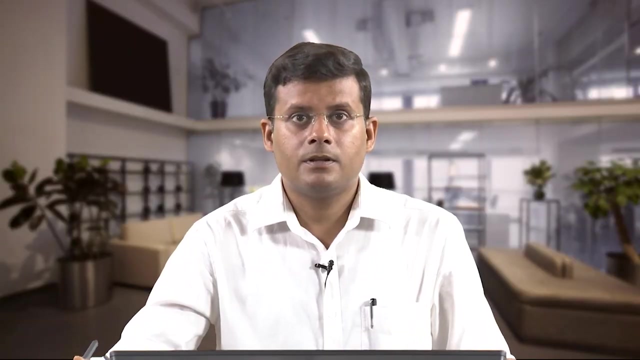 Okay, People sign the object and the light. after getting scattered from the object and a reference beam, They all fall on a photographic plate and they interfere there And this is recorded on the photographic plate. Okay, So the photographic plate is recorded on this plate and this plate thus becomes a hologram. 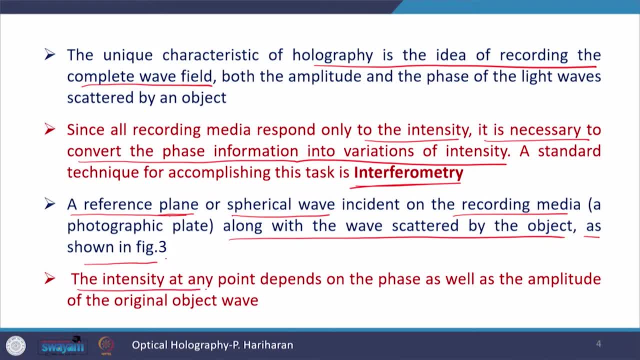 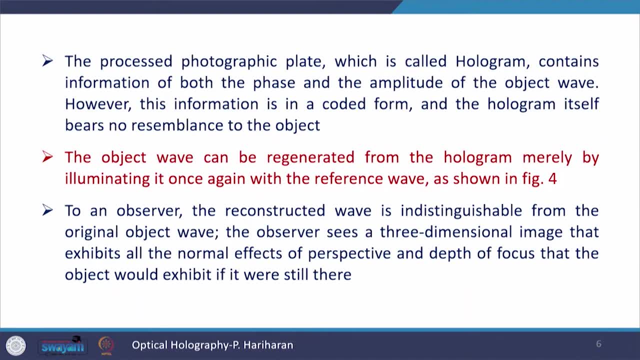 And this is what is written here. The intensity at any point depends on the phase as well as amplitude of the original object wave. Now the processed photographic plate, which is called hologram, contains information of both the phase and the amplitude of the object wave. 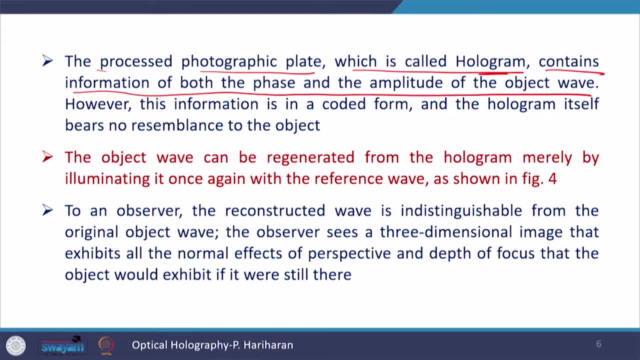 Because now it is an information of the phase and the amplitude of the object wave- Okay, Okay- interference pattern which is getting recorded. Therefore, both intensity and phase is being captured by this holographic plate, or hologram. However, this information is in coded form. 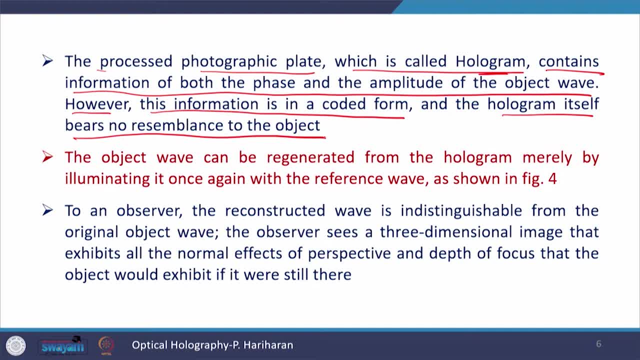 and the hologram itself bear no resemblance to the object. It is not like one to one correspondence between a holographic plate or hologram with the object, as we expect in a usual photo. If a person is standing here and we have the photograph of the person, then we can easily. 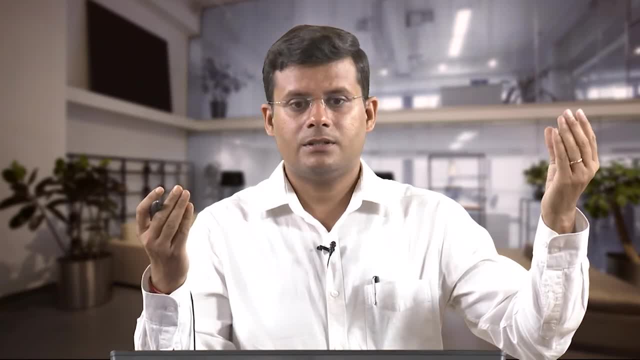 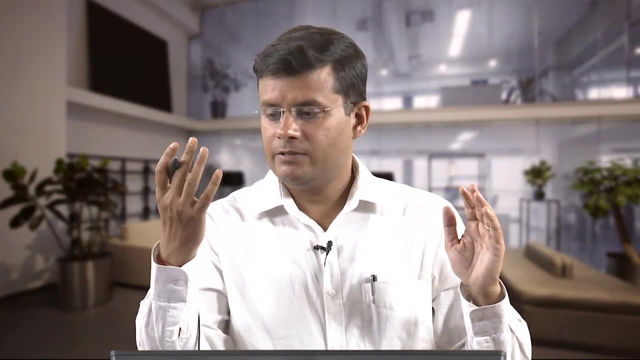 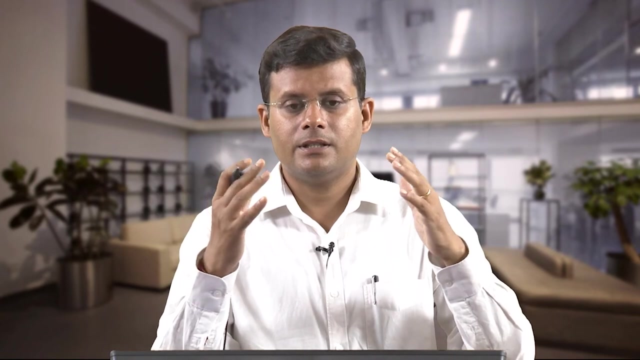 match the two and say that this photo resembles the object or the person who is standing here. But in case of a hologram, the hologram is coded in such a way that if you see the hologram and the object then you will say that there is no resemblance. The hologram does not correspond. 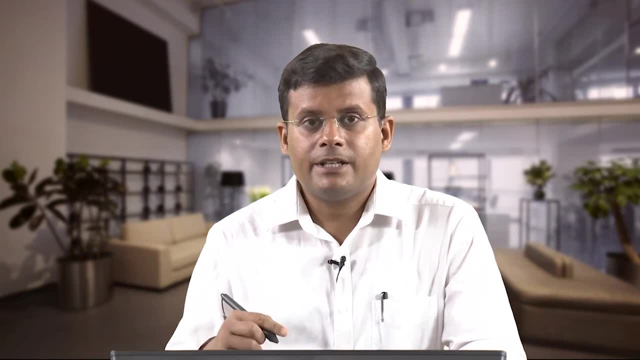 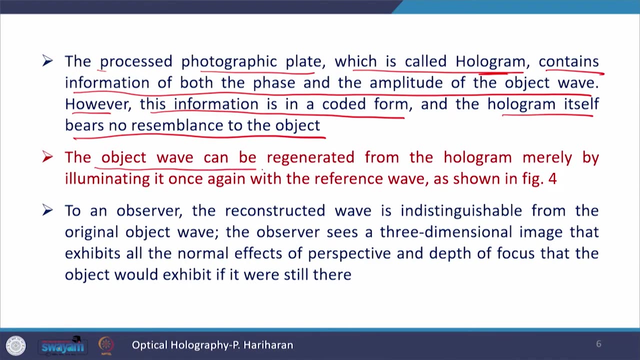 to the object. okay, And there are some specific techniques to generate the image of this person with the object from this hologram. Now, the object wave can be generated from the hologram merely by illuminating it once again with the reference beam, as shown in the figure 2.. Let us go back to the figure. 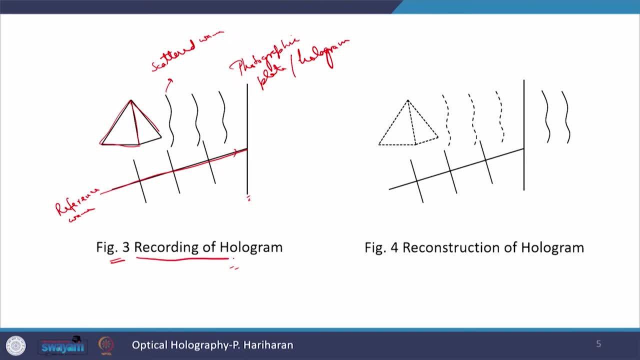 In figure 3, we understood the recording of hologram. We put a photographic plate here and then we illuminated the object. Okay, We put the object and then the scattered light from the object, it falls on the plate and, as well as a reference beam, also falls in this plate. These two beams, they interfere. 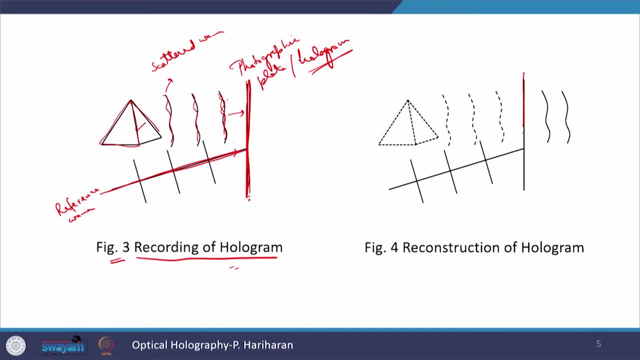 and they create a hologram. Now, this is our hologram and using which we want to reconstruct the object here. This is hologram. Now, to do this, we will use the same reference beam, This one. okay, We illuminate the hologram with the same reference beam and then, after, 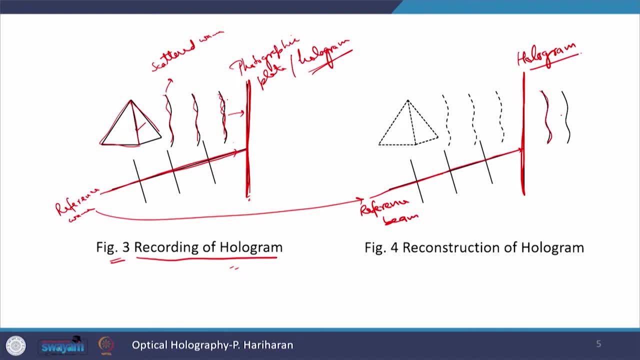 the illumination of some scattered light will pass through this hologram And if you look from this direction, then you will see the virtual image of object appear here floating in air. Okay, We will use this hologram to recreate the larger source of light. This giving us the image of instance, profitable once we perform a photograph with the object object. So this will create a hologram and once through that you will be able to see that the object is visible into the mirror. Okay, In the preference beam will appear, some scattered light pass through this hologram and if you look from this direction, you will see virtual image of object appear here floating in air. 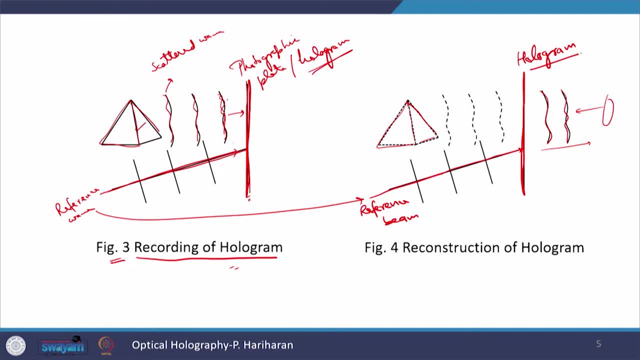 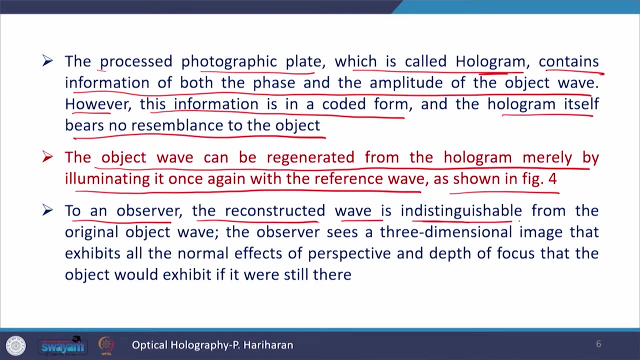 And this virtual image is a 3D image. it have the perception of depth now, because phase information is also embedded there. Now, to an observer, the reconstructed wave is indistinguishable from the original object wave. The observer sees a three-dimensional image that exhibits all the normal effects of perspective. 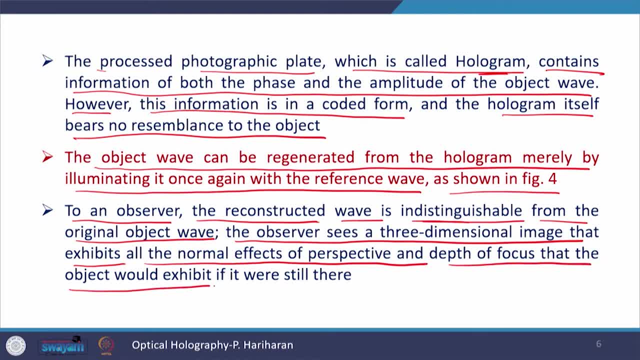 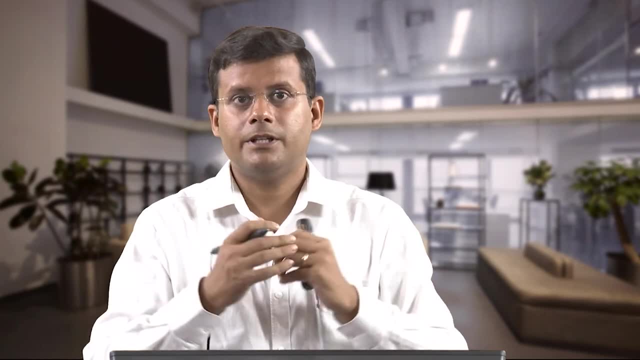 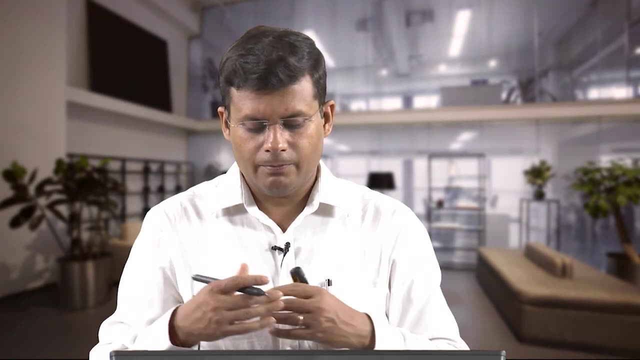 and depth of focus that the object would exhibit if it were still there. The constructed image of the object would completely resemble the original object and it would be in 3D form. it would have the perception of depth. It will have all the normal effect of perspective and depth of focus. 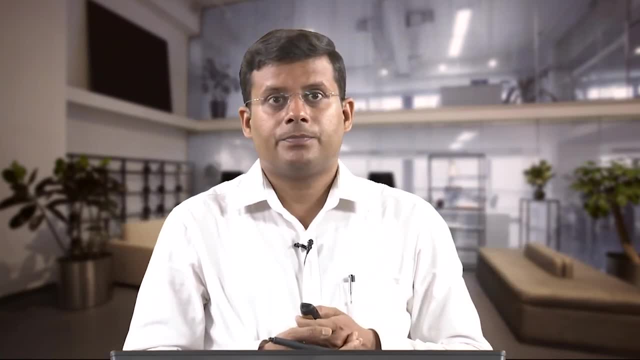 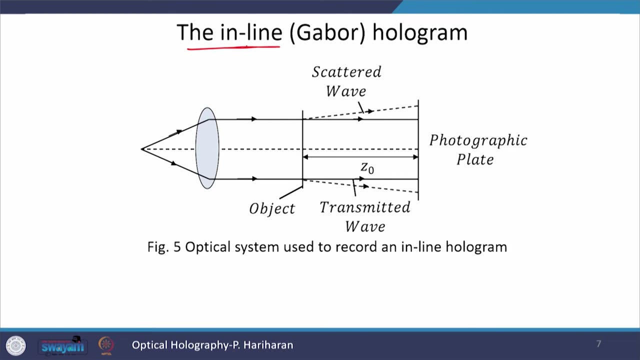 Now, this is the beauty of holography. Okay, Now there are several ways of recording and reconstructing the image in holography. Now, one of the way is inline hologram. An inline hologram was proposed by Gabor. 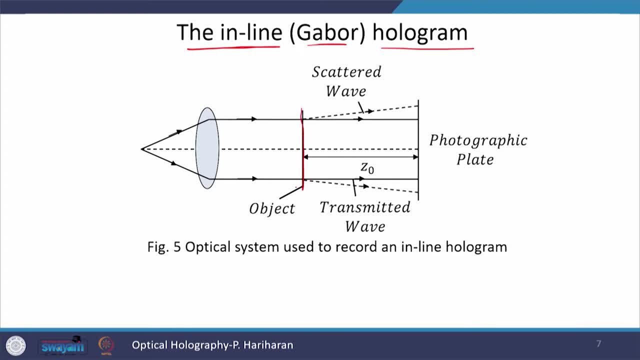 Here. what he did is that he picked some object and he put a photographic plate coaxially with the object And then he illuminated it. He illuminated the object with a light source using a lens coaxially, and then what happens is that when light falls on this object, then a part of the light get transmitted, while 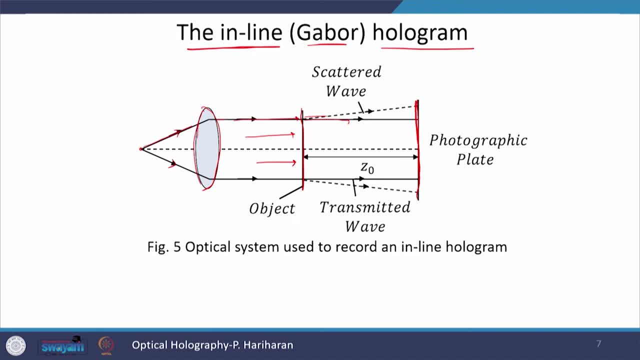 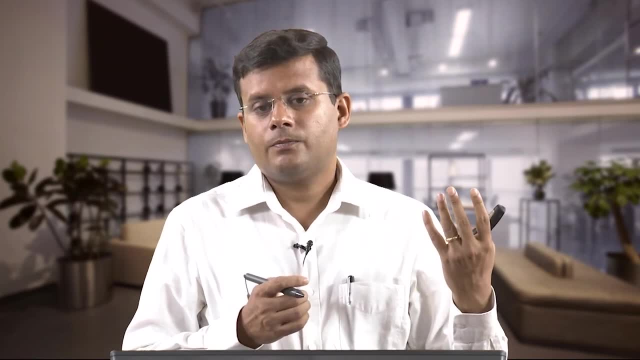 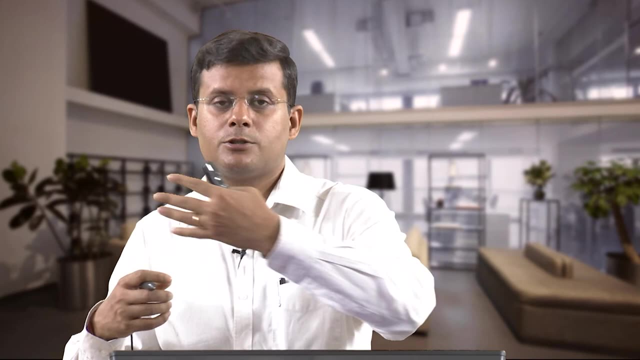 a part, get scattered. Why? Because in this inline hologram, the object is chosen to be semi-transparent. Okay, Therefore, wherever the light get hindered, it get scattered, And if there is no obstruction in the path of the light rays, it passes through smoothly. 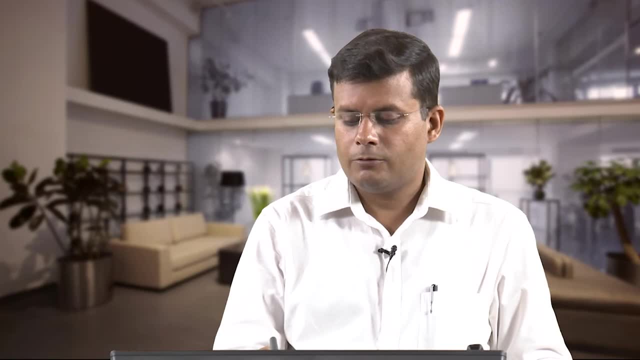 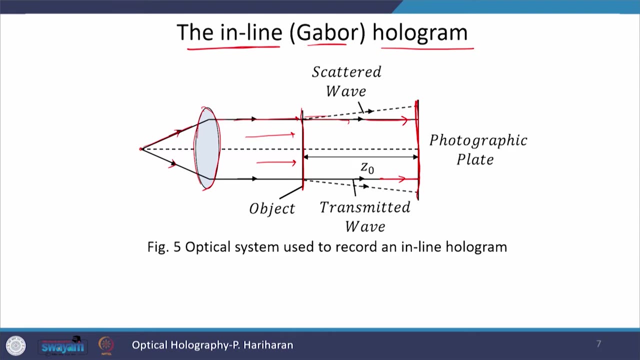 It passes through untouched and therefore the direct light which is received on the photographic plate can be treated as reference beam, while the light which got disturbed due to the presence of this opaque portion on the object plane, it got scattered and therefore on a photographic plate this is scattered. 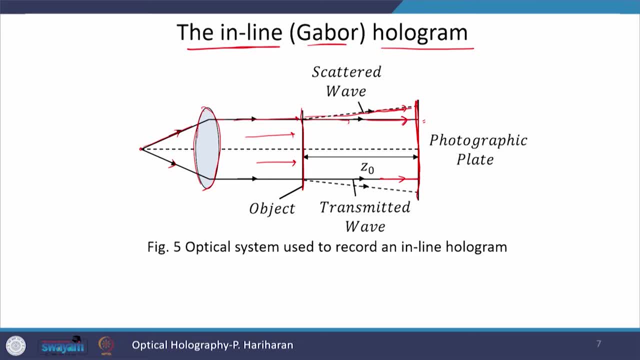 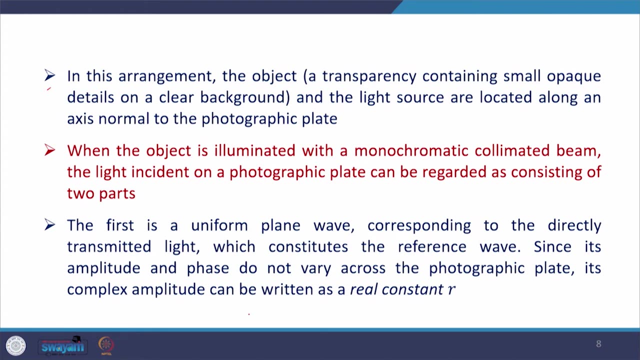 Okay, And the reference beam. they interfere and form hologram. Now you see that all these things are coaxially placed in this schematic picture. Therefore, this type of hologram is called inline hologram, And the explanation of this inline hologram is written here, which says that in this arrangement, 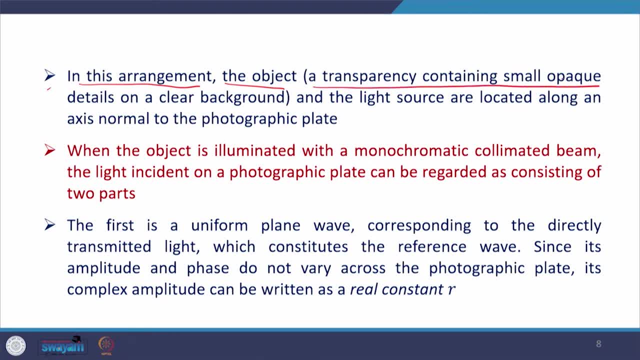 the object, which is a transparency containing a small opaque details on a clear background, and the light source are located along an axis normal to the photograph. When the object is illuminated with a monochromatic collimated beam, the light incident on a photographic plate can be regarded as consisting of two parts. 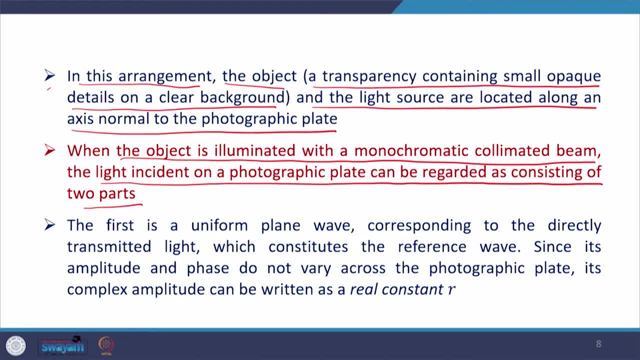 What are those two parts? The first part is a uniform plane wave corresponding to the directly transmitted light, which constitutes the reference wave, Since its amplitude and phase do not vary across photographic plate. It is a complex. amplitude can be written as a real constant R. Do remember it. 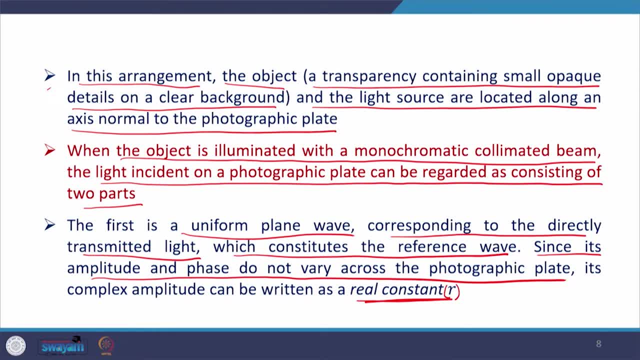 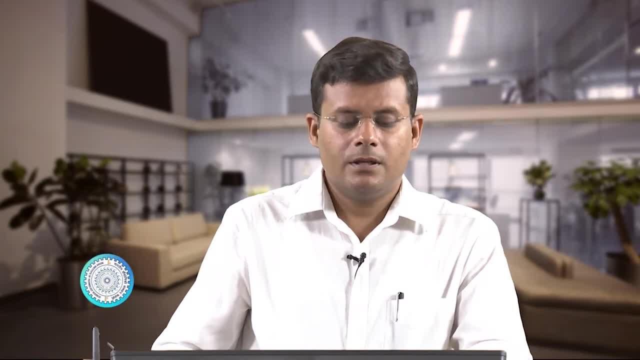 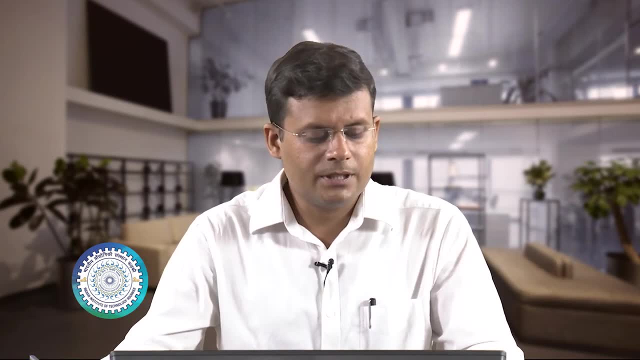 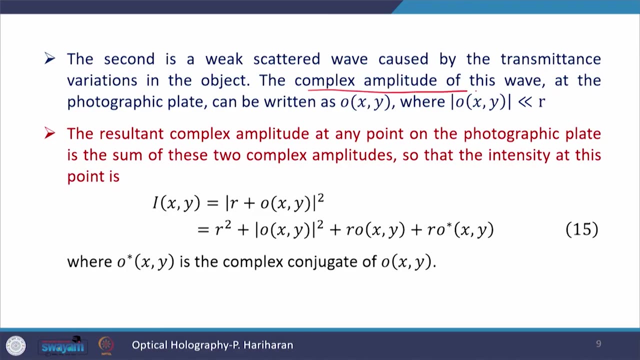 The amplitude of the undeviated light or the reference beam, is represented by real constant R- It is not complex- while the second part, which is the weak, scattered wave that is caused by the transmission variation in the object, It is complex. Okay, And the complex amplitude of this wave at the photographic plate can be written as O. 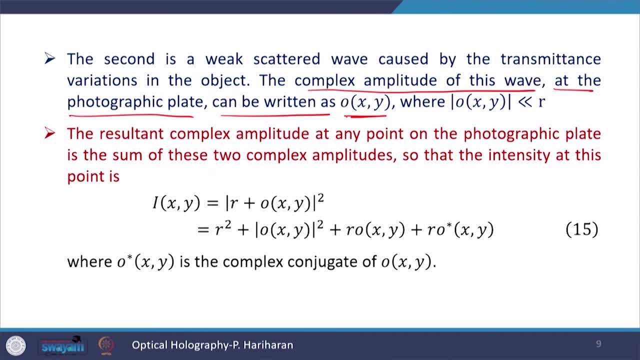 function of XY, because the variation is in the transverse direction. in the Z direction it is a propagation happening. Okay, And since the scattered wave is of weak amplitude, mod of OXY would always be much, much smaller than R. the contribution from the reference beam. 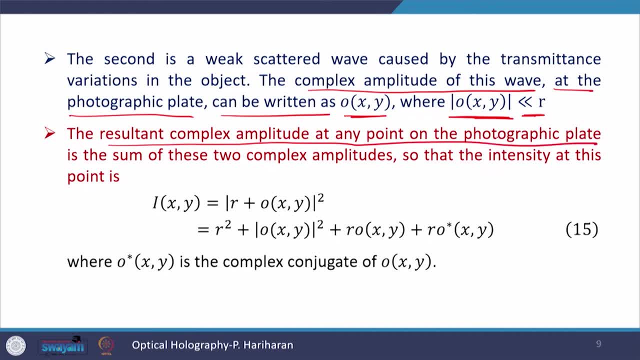 Therefore, the resultant complex amplitude at any point on the photographic plate is sum of these two complex amplitudes. The superposition principle is applied here. Therefore, the intensity at the at any point on the screen on the photographic plate would be the contribution from the reference wave plus the contribution from the scattered wave. 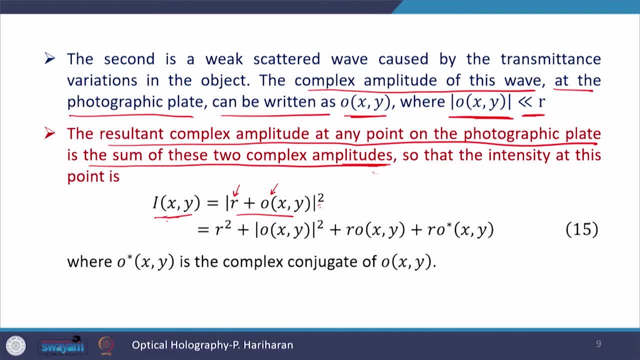 added and then squared. This would give the intensity. If you expand it, then we will get R square, then mod of O square, then R into O and then R into O star. Okay, Since R will, Since R is a real number. therefore, the complex conjugate of R would be equal to R and therefore, 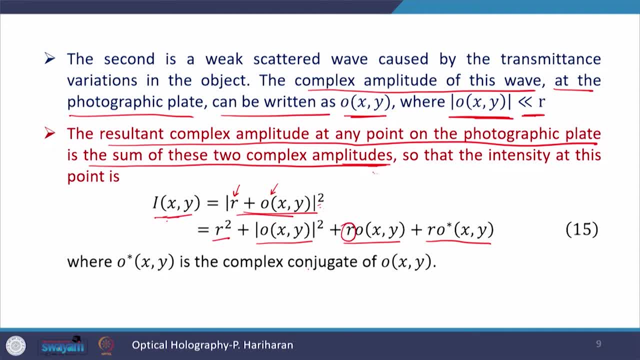 though no star sign is there here on top of R, But O is a complex. therefore there is O star term here in equation number 15.. This is the resultant intensity which photographic plate will receive. Now a positive transparency is met from this recording. 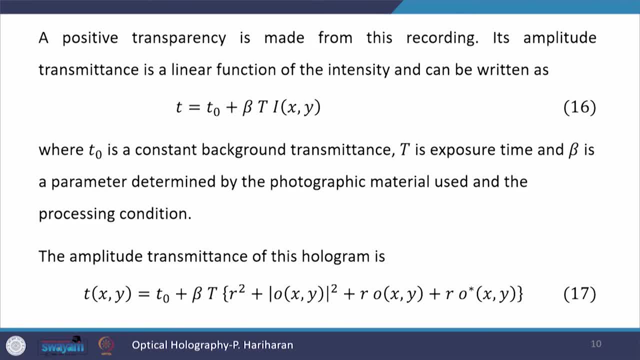 Its amplitude transmittance is a linear function of intensity and can be written as this: that the Amplitude transmittance T of this positive transparency would be equal to T naught into beta capital, T into I. I is the intensity which was received at the photographic plate. 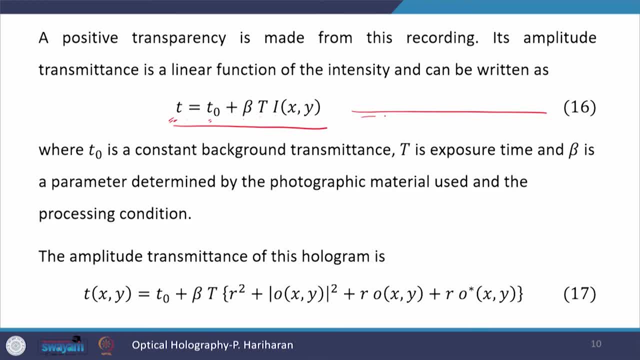 Now we know that in holography we now launch reference beam on the hologram to reconstruct the image. Amplitude transmittance through this hologram is given by equation number 16, where T naught is a constant background transmittance, T is the exposure time. 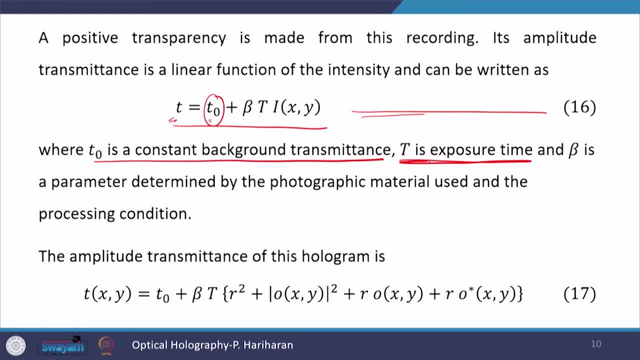 Which means how long the photographic plate remained exposed. And beta is a parameter determined by the photographic material used. okay, because the material also play a role And it also depends upon the processing condition, how the photographic plate is processed. okay, The amplitude transmittance of this hologram. 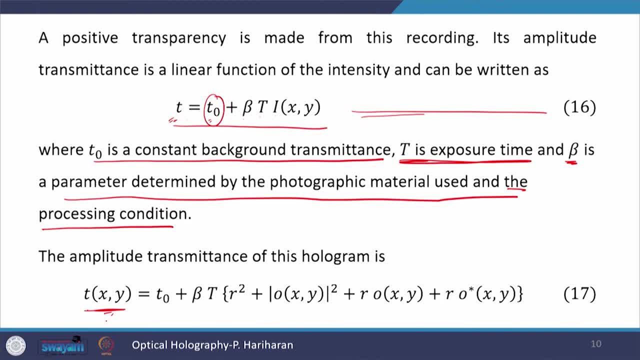 Therefore, We Are given by this expression where we have just replaced this I, which is intensity which is recorded at the photographic plate, by equation number 15.. We substituted the expression of 15 there. okay, After substitution we get this big expression. This is amplitude. transmittance of hologram. 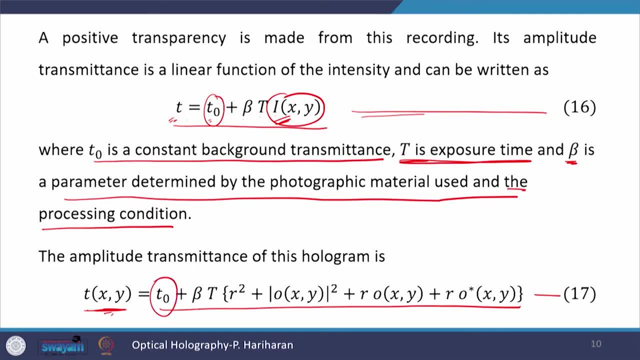 Now you see here this T naught is the background term, and then we have this term and this second term, third term and fourth term, And this term is O square term. Okay, And O is already very small. therefore, O square would be very, very small, which can easily. 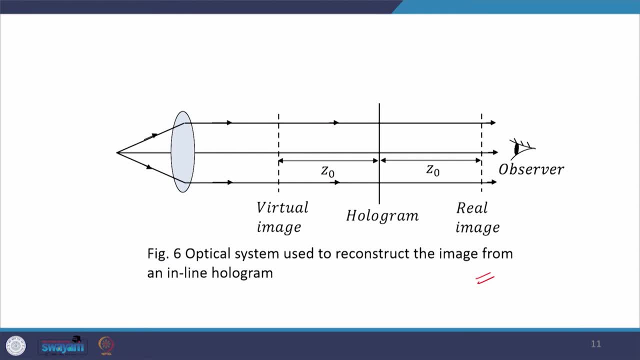 be neglected. okay, In inline hologram the reconstruction process is shown here schematically. Here in: what we did is that we place hologram here and then we shine the light and everything is coaxial, as system name is inline hologram and observer looks into the hologram from. 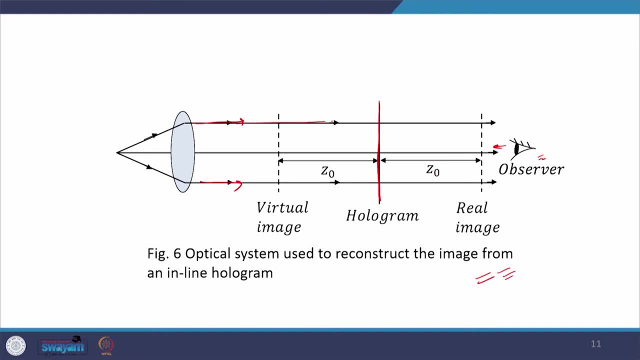 this direction. Now you see that when light falls on the hologram, then one of the image is created here, while the other image is created here. This image, which is created at the backward direction, at z naught distance, is called virtual image, while the image which is created in the forward direction, which is close to the 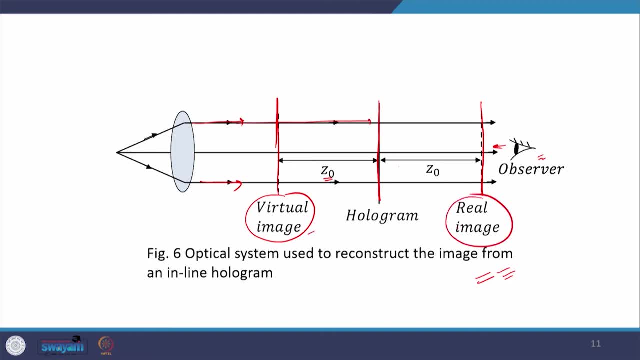 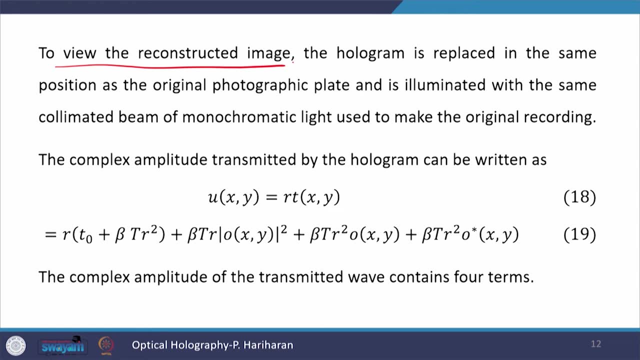 observer. it is called real image. We will learn about this virtual and real image in the forthcoming slide. now. Now to view the reconstructed image, The hologram. Okay, The hologram is replaced in the same position as the original photographic plate- The photographic plate now termed as hologram- and it is then illuminated with the same collimated. 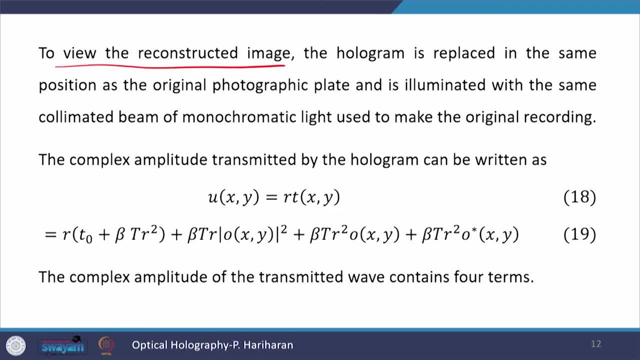 beam of monochromatic light that was used to make the original recording. Okay, The reference beam should be the same. Now the complex amplitude transmitted by the hologram. it can be given by equation number 18.. This is the complex amplitude which is transmitted through the hologram. 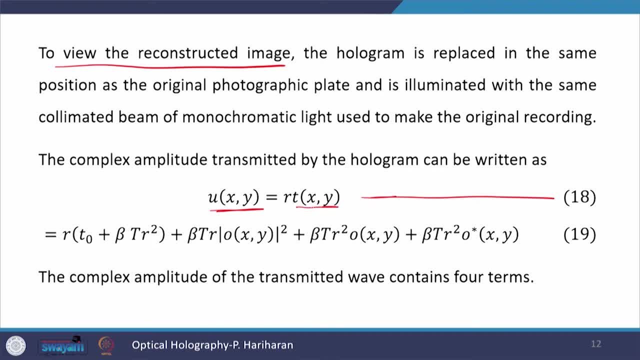 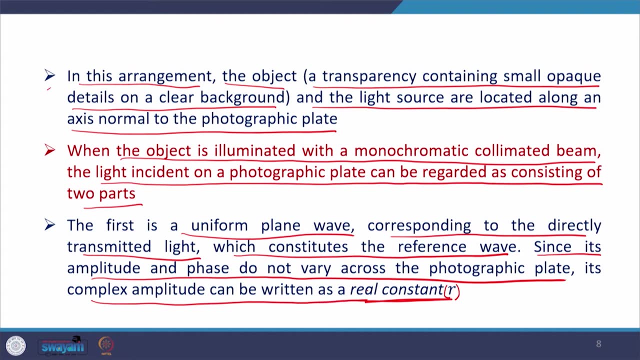 Okay, T is the amplitude, transmittance, and then it is multiplied by R. Why R? Let us go back and remember what R is. R is nothing but the complex amplitude of the light which passed through the semi-transparent object, which remain unaltered. 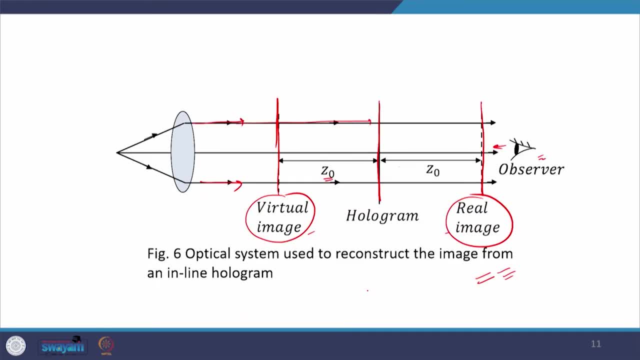 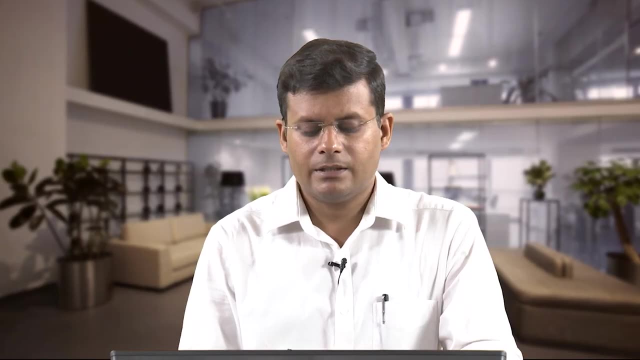 Okay, Now here too we are signing the hologram with the light. Okay, And the part of the light will get transmitted. Okay, The transmitted part would be given by R into T. Okay, This is the amplitude of the reference wave, and then this amplitude is multiplied by the. 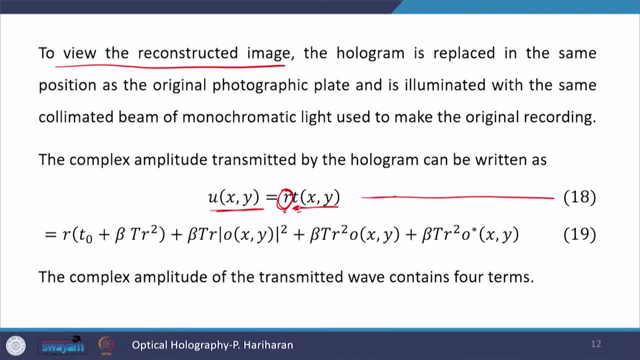 amplitude transmittance function to get the exact value of the amplitude at the transmission end. Now we will substitute for small t and after substitution we get this big expression. Okay, The complex amplitude of the transmitted wave contains four term. Okay, This is our first term. 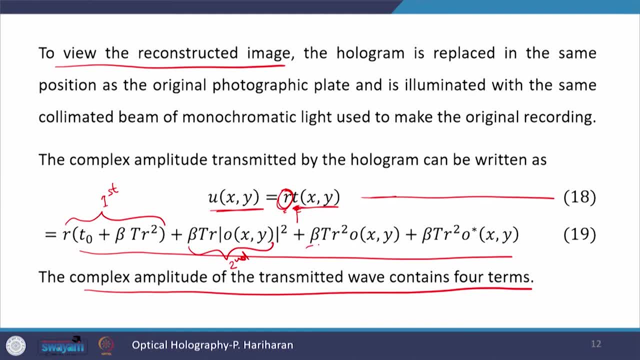 This is our second term, This is the third term and this is the fourth term. Now, in the first term, we see T, not beta capital, T R. Okay, R is also here, But O is not appearing here, And O is contribution from the scatter. 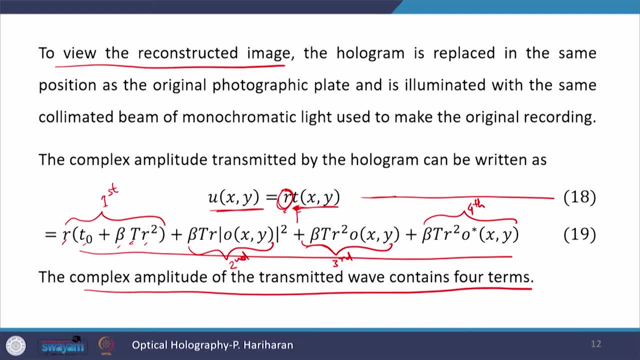 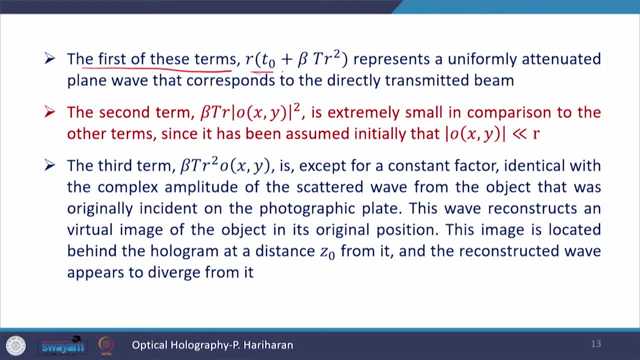 Okay, It means: object: information is not there in the first term. Okay, And this is what is written, The first term of these terms, which is this: This represents a uniformly attenuated plane wave that corresponds to the directly transmitted beam. Okay, 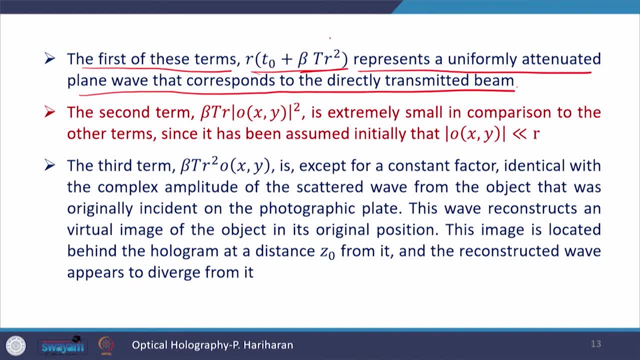 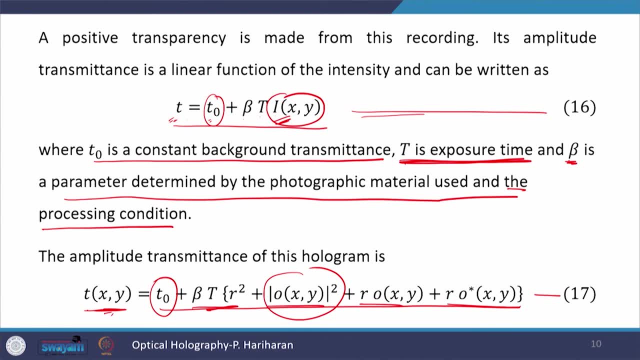 Beam is coming, It is getting directly transmitted. R is amplitude of the reference wave, T not is the background transmittance, T is the exposure time And beta is the parameter determined by the holographic material and the processing condition. Okay, 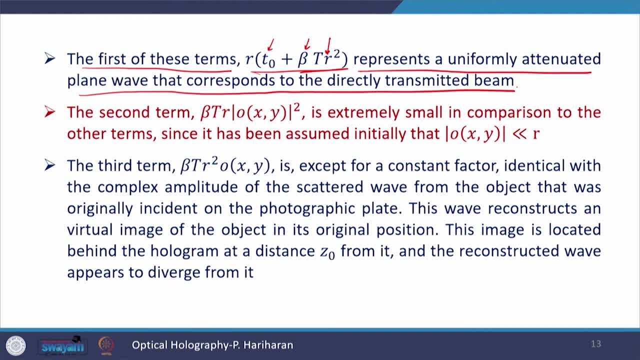 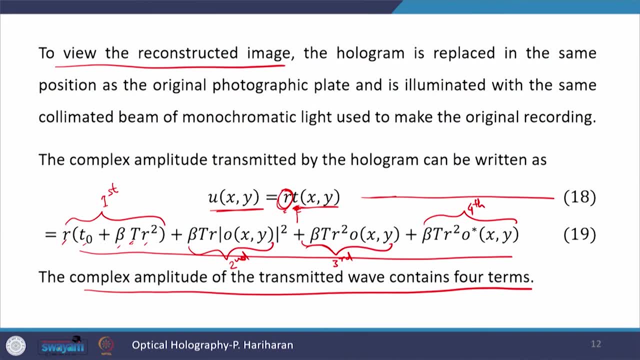 Therefore the object information is not here in the first term And therefore it corresponds to the directly transmitted beam. It has nothing to do with the reconstruction. Now let us go to the second term. The second term is O square term, which I said already. it is very small. 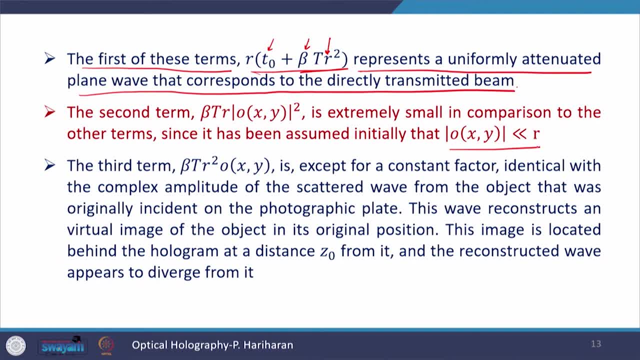 Therefore it can safely be neglected, because O is already much, much smaller than small R. Okay, So T? R square O is, except for a constant factor, identical with the complex amplitude of the scattered wave from the object. Okay, And that was originally incident on the photographic plate. 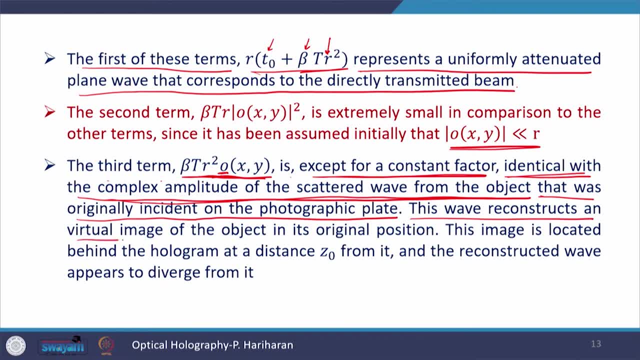 Now this wave reconstructs a virtual image of the object in its original position, And this is the virtual image which appears here. Okay, This image is located behind the hologram, at a distance z, not from it, and the reconstructed wave appears to diverge from it. 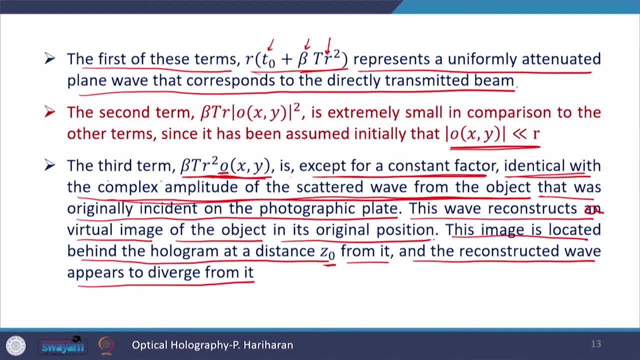 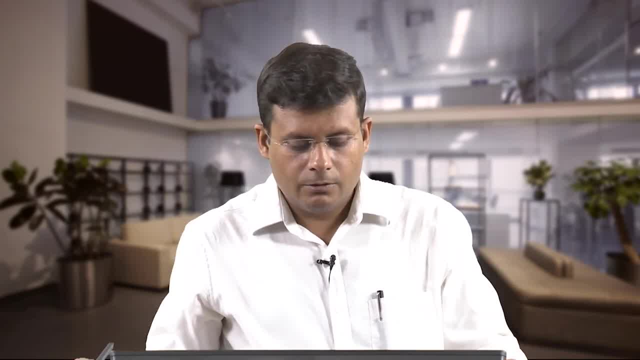 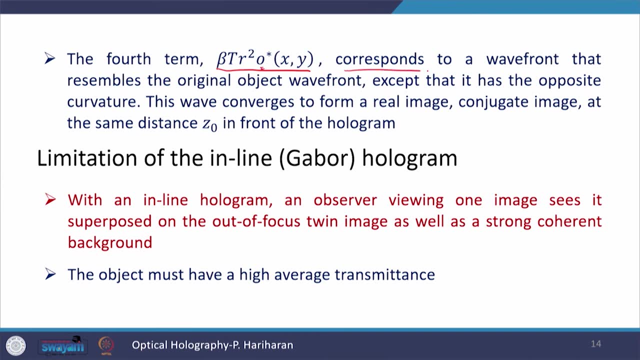 It diverges if you move away from the hologram. then the reconstructed image diverges. It becomes bigger and bigger if you move away from the hologram. Now the fourth term is beta, T, R, square, O star. Okay, This is a complex conjugate of O. This corresponds to a wave front that resembles to the original. 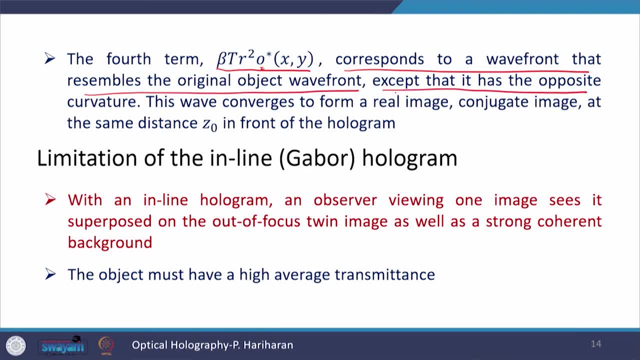 object: wave front, except that it has the opposite curvature. because of this complex conjugation, The wave converges to form a real image, which we also call a conjugate image, And this image is formed at a same distance, z, not in front of the hologram which we call. 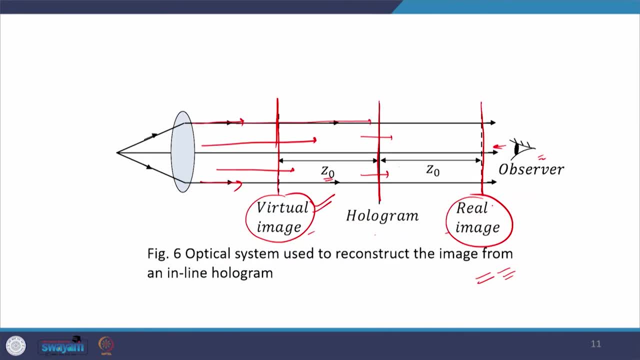 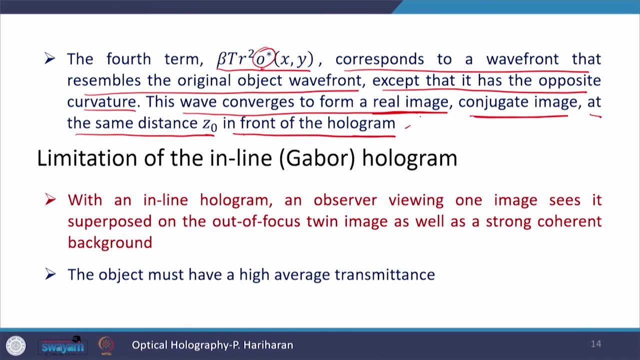 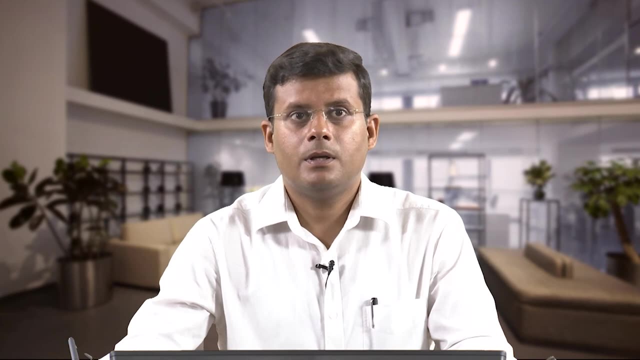 the real image. Okay, This is the first term which is shown here. Now, this is how, in in-line hologram, we get two images, one virtual and one real. But associated with this in-line hologram, or Gabor hologram, there are a few limitations. 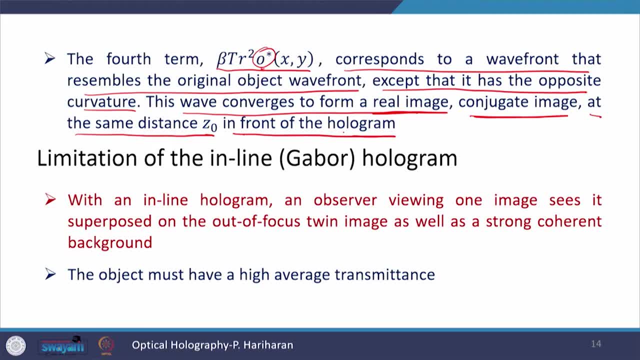 which is very much obvious. The first limitation is with an in-line hologram. The first limitation is with an in-line hologram. The first limitation is with an in-line hologram. So with an in-line hologram, an observer viewing one image sees it superimposed on. 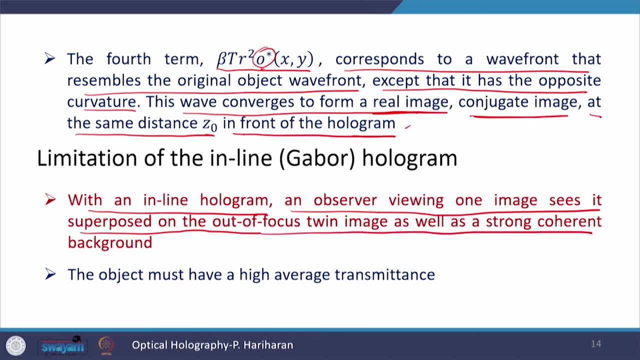 the out of focus twin image, as well as a strong, coherent background. Why, Let me repeat it, With an in-line hologram, an observer viewing on image sees it superimposed on the out of focus twin image, as well as a strong, coherent background. 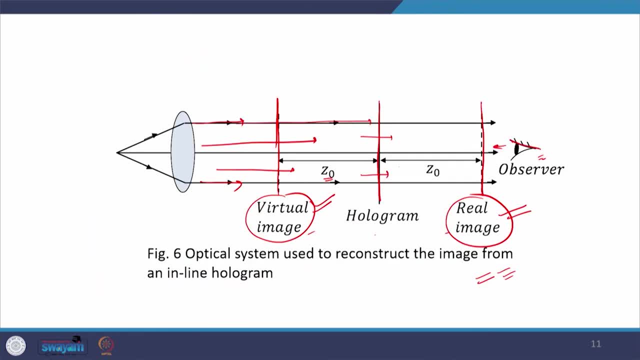 Okay, Which means the observer which is viewing from here. it says this image as well as the second image. The two images are being simultaneously watched and, apart from this, you are also seeing the rays from the source coming to the observer. Therefore, it is very difficult to make out. 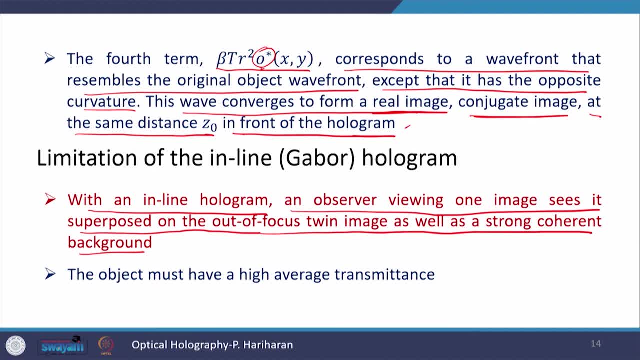 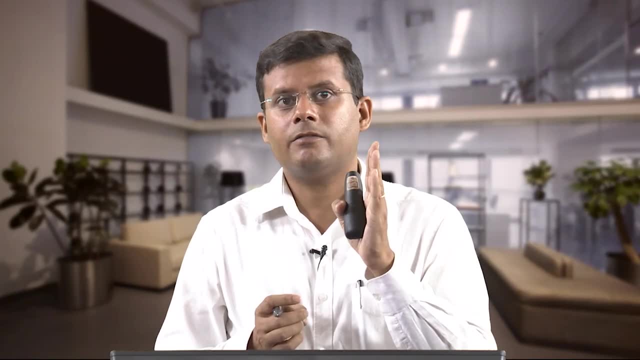 the image properly, because in our field of view there are several things which are appearing simultaneously. The second thing is that to create a hologram using inline technique, we require an object which must have some transmittance. We cannot use an opaque object. 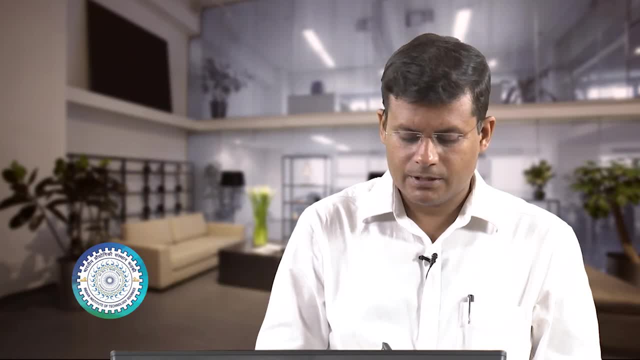 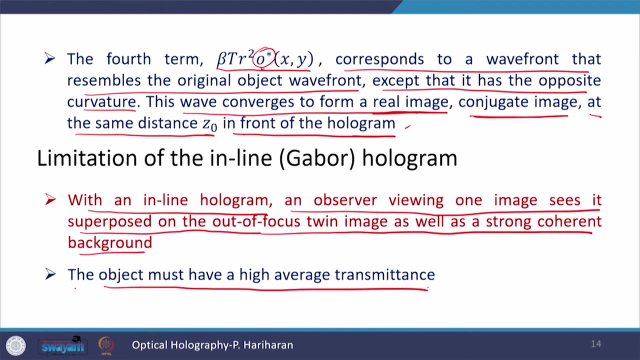 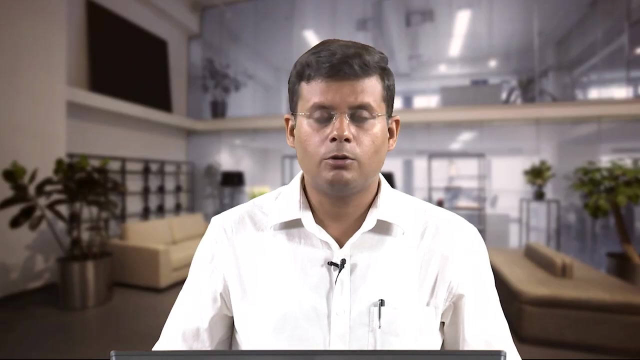 here. This is the second limitation. It is limited to some semi-transparent object. An object must have a high average transmittance to enable this technique to form a hologram here. Now this is all about inline hologram, and in the next class we will talk more about. 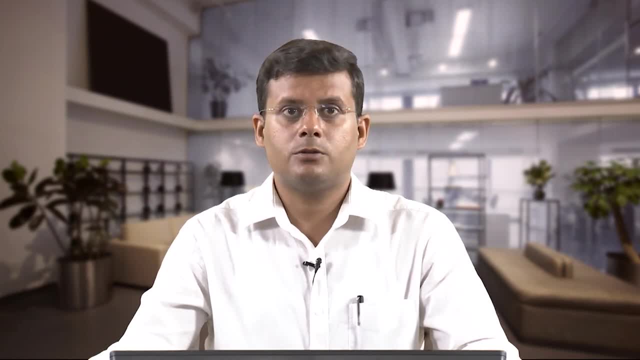 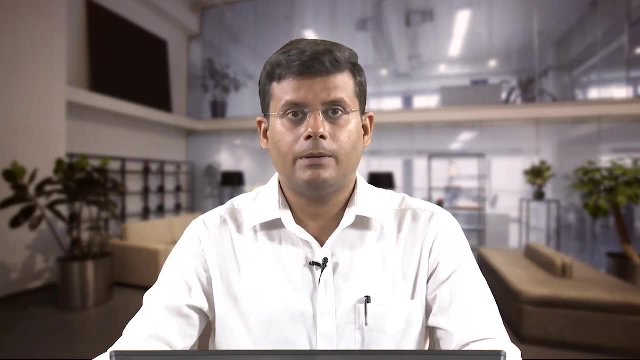 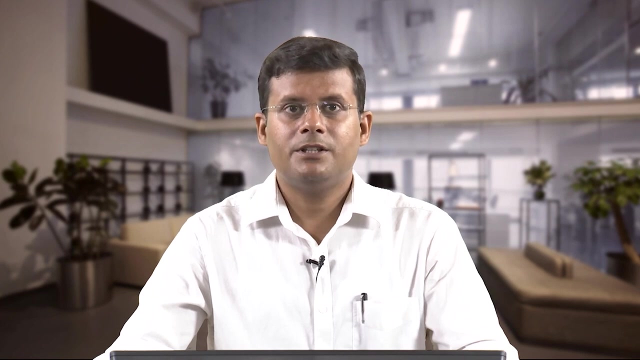 holography- and we will learn about off-axis hologram also- which removes these two limitations which are imposed in inline hologram. With this, therefore, I end my today's lecture and thank you for joining me. See you in the next class. Thank you.